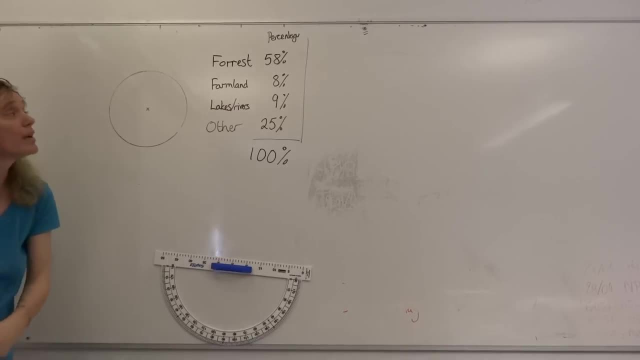 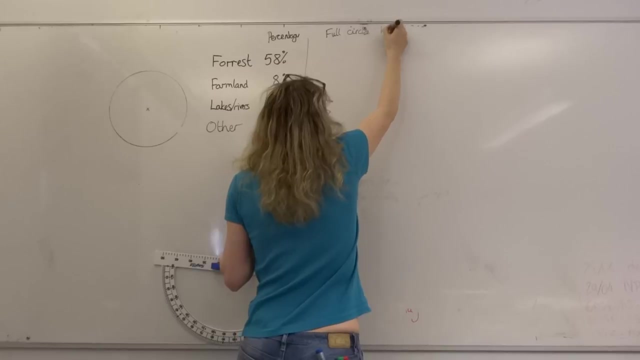 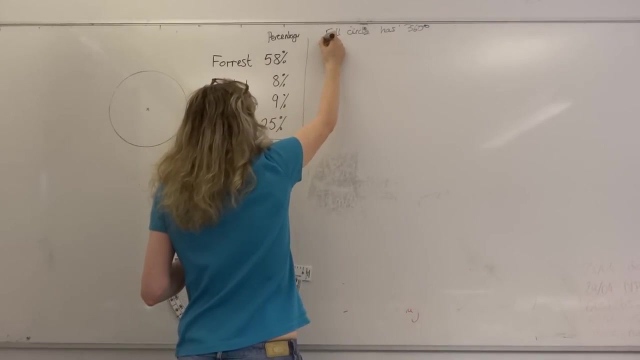 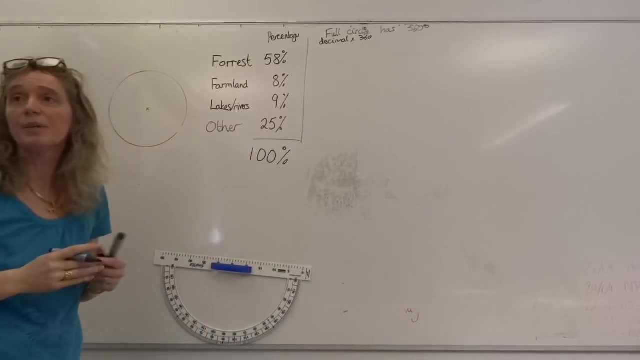 to fill this with a hundred percent, we'd have 360 degrees. so our full circle has 360 degrees. so 58% of our circle would have the percentage as a decimal multiplied by what we would have in 360 if it was a full circle. so a hundred percent would have 1 times 360. that would be 360 degrees. so forest will. 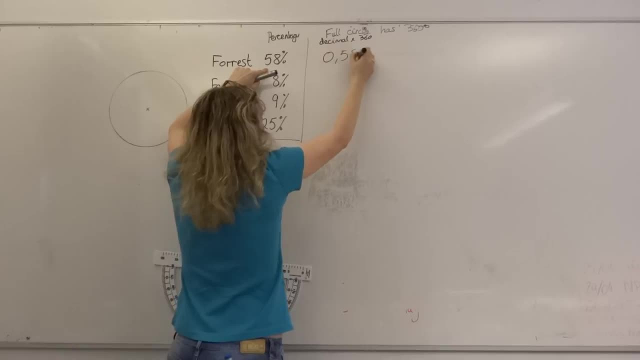 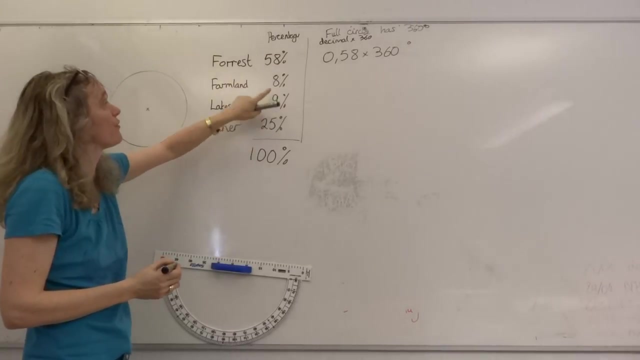 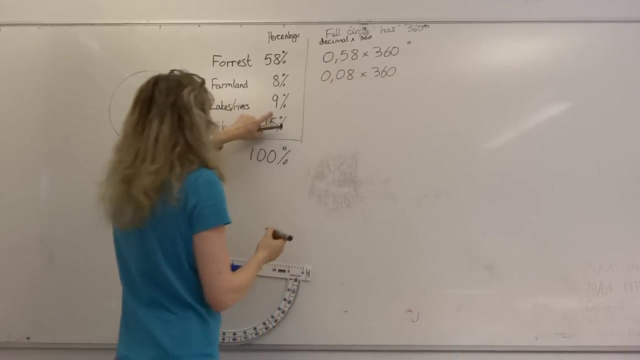 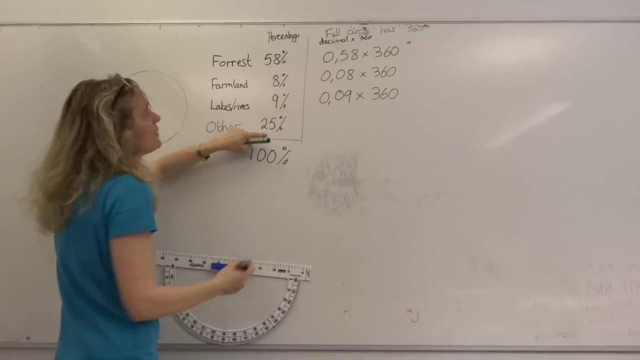 have 58% as a decimal, that's 0.58 multiplied by 360 degrees. that would give us how many degrees we should be able to convert into a pie chart. if we were to go around the whole circle we'd have. we should represent the forest as 8% as a decimal is 0.08 times 360, 9% is 0.09 times 360 and 25% is. 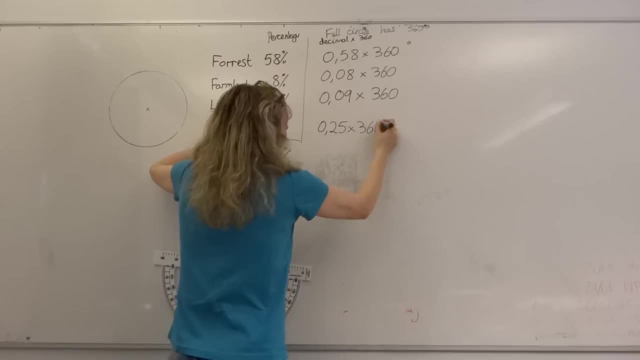 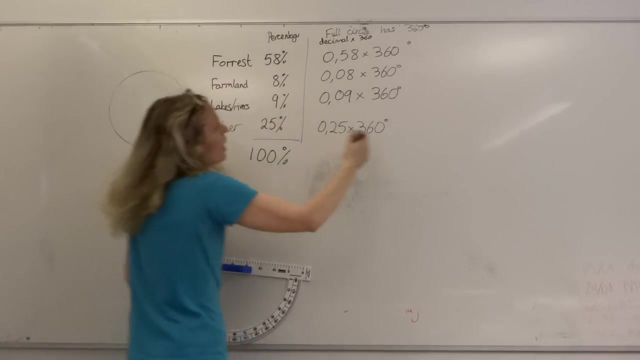 0.25 of 360 degrees. but we know that 0.25 or 25% is just a quarter a quarter of a circle we know is 90 degrees 360 divided by 360 degrees. so we know that 0.25 or 25% is just a quarter a quarter of a circle we know is 90 degrees 360 divided. 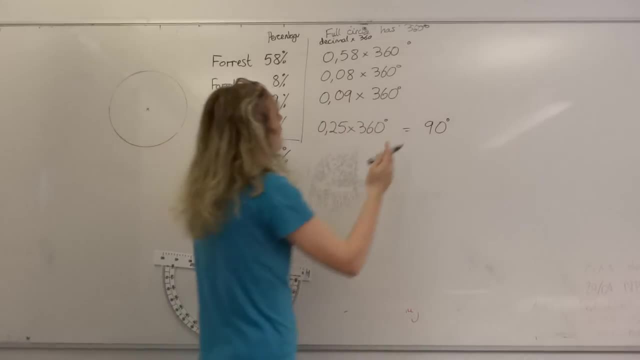 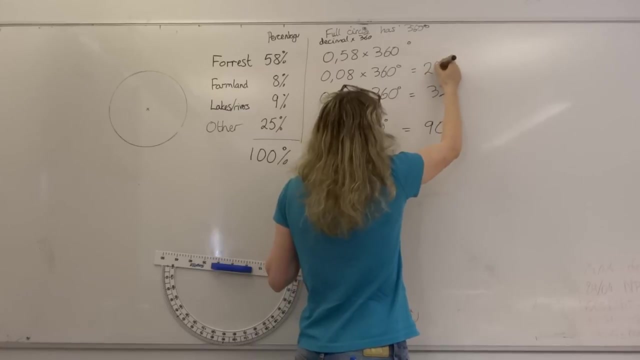 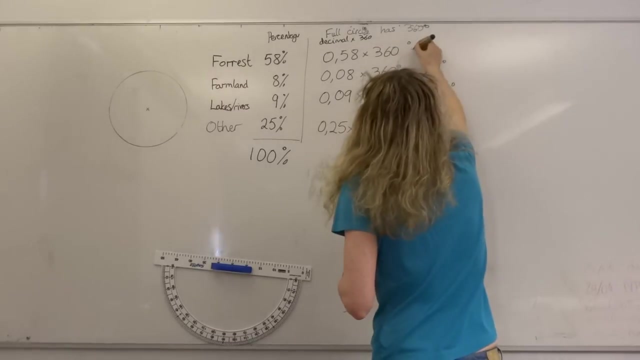 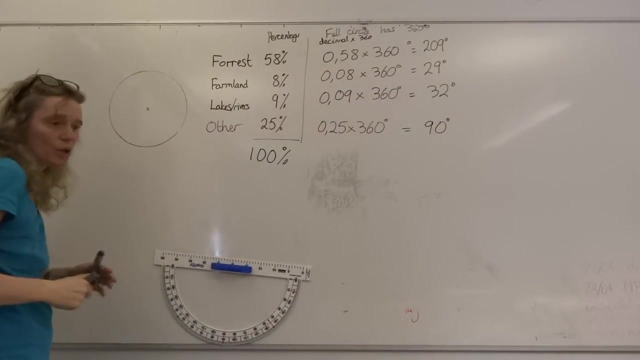 4 is 90, so that was nice and easy. point 09 is 32 degrees, point 08 is 29 degrees involved and 58% is 209 degrees. so now we know what degrees we need to draw on a circle, and we usually use color pens. 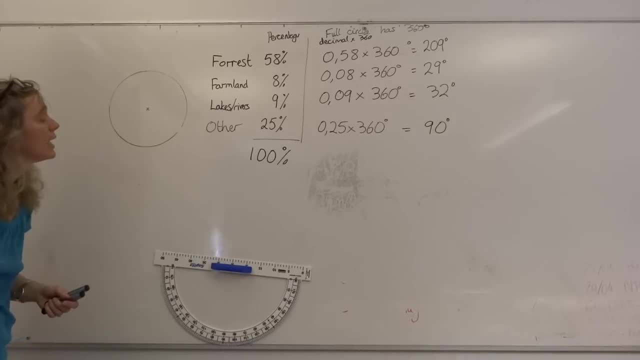 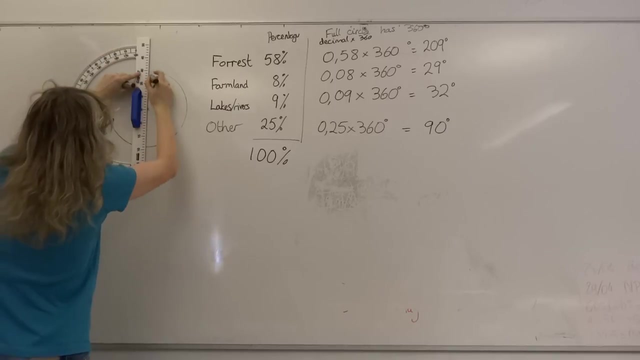 for the different colors will do that as well as an end. let's Let's start with the easiest one, which is our other. the 90 degree angle is nice and easy to draw. Start with drawing a vertical line. so this is the start of our circle, from the top down. 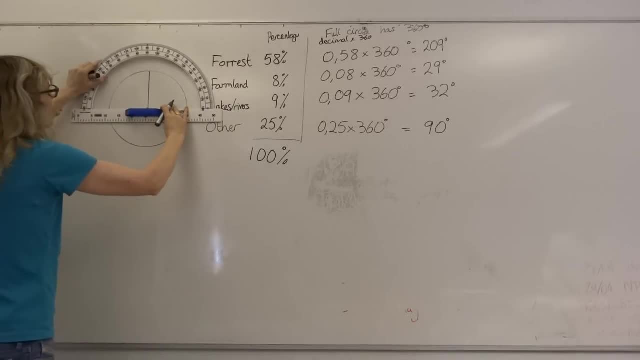 Now we need a 90 degree angle. so we start here using our protractor. Make sure that we're in line. Let's extend this line up so we actually see where is our starting point. So we get the starting point on the protractor. nice and clearly. 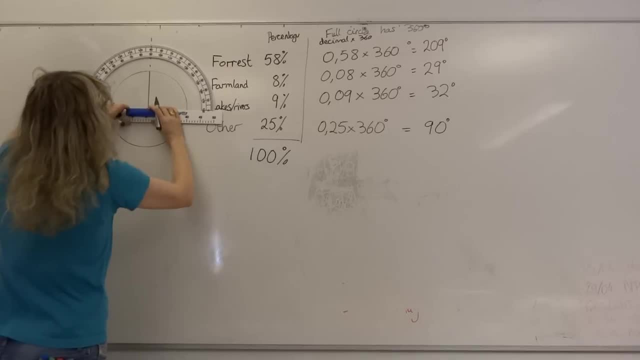 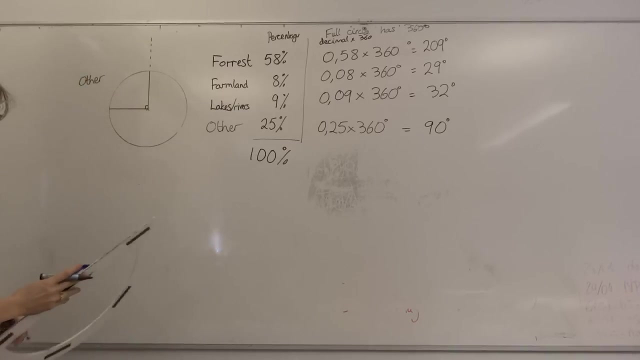 Put our centre point against the middle point of the protractor and draw 90 degrees, which is out here. So here we have our perpendicular 90 degrees. this is our other. From that we need a 32 degree angle. So we put our protractor at the end of the forehead. 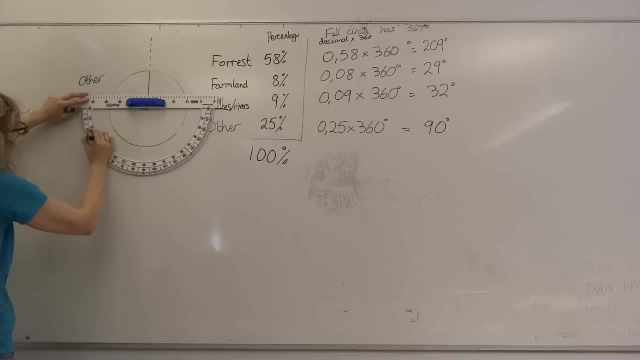 This is our first mark- and go down 32 degrees- 10,, 20,, 30,, 2, which will give us a line, And we don't need to draw the line all the way out here to the dot, we just take it to. 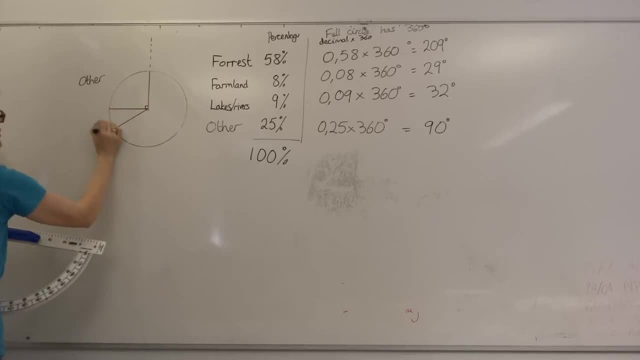 the end of the circle. This is our lakes and rivers at 9%. We now want a 29 degree angle from that, so we put our protractor at the right point with the centre point here from the protractor in the middle point of the circle. 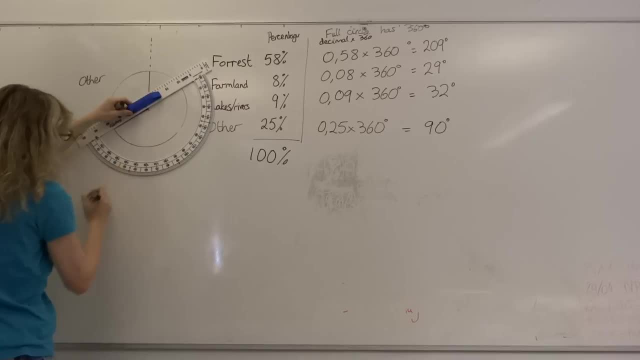 and we go around 29 degrees, which would be here, and we draw our line out to that point: 29 degrees here, and that is our farmland, and if we've done everything correctly, we should have first 180 degrees plus how many more degrees do we have to add on to that? 180, 190, 209 degrees, and this is our forest. 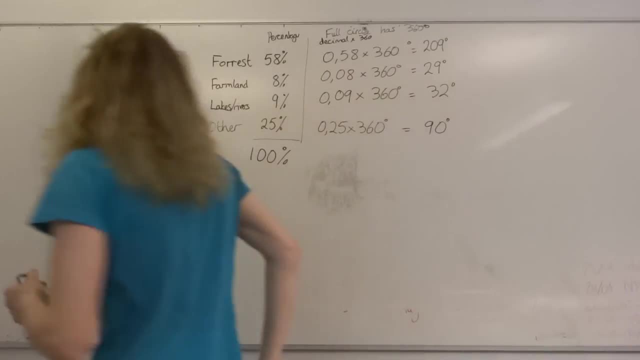 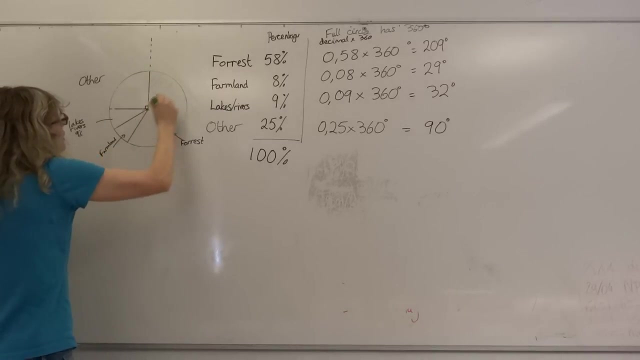 so to finish off, a pie chart and all nice and neatly, at the end we give each of them different colours. it seems sensible to have our forest, as being green makes a pie chart very easy to read with the colours there. so, for example, if you look at the green dash, you can see that the forest is represented by a green dash. 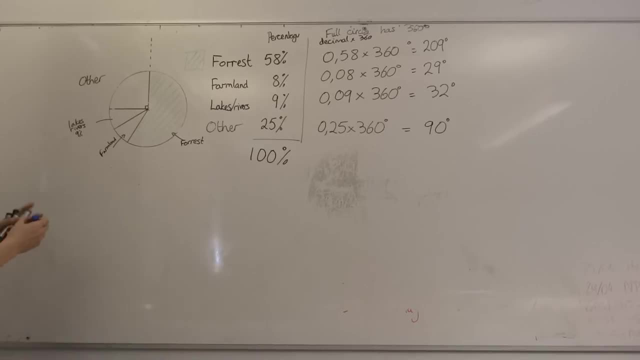 what about our farmland? we'll colour that blue and represent that here, although it would have been more sensible to have the lakes blue. sorry, lakes are going to be black, which is maybe what they'll end up being if we don't actually start improving on how we take care of them.